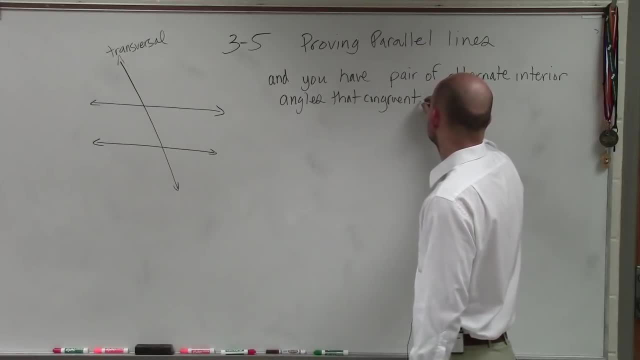 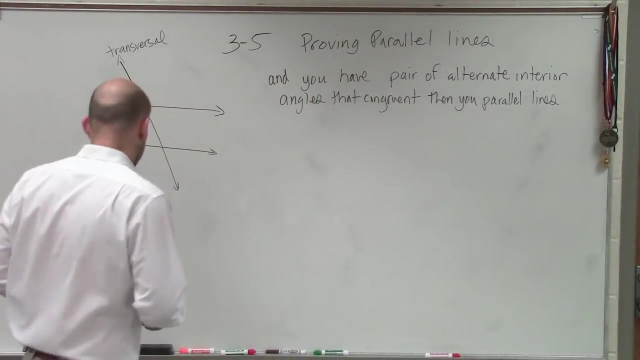 in measure, then you have parallel lines. Okay, So what I'm trying to say by that is: let's say I have these two lines right Now. let's say I give you a case of alternate interior angles. Let's say I say this is 75 degrees. 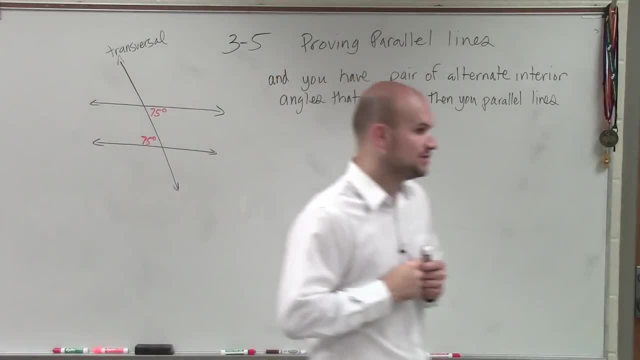 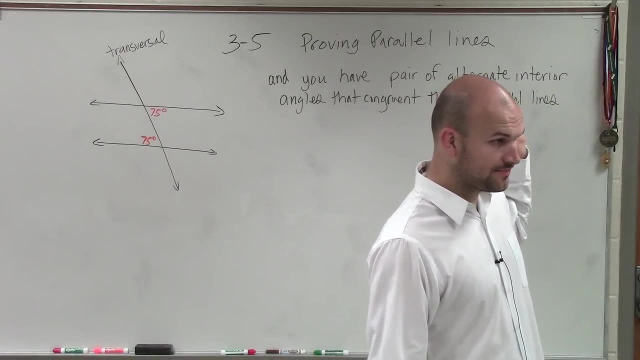 and this is 75 degrees. All right, Virta, can you confirm those are alternate interior angles. Yes, Kim, would you say those are the same measure? Would you say those are the same measure? So, since I have a pair of alternate interior angles that are the 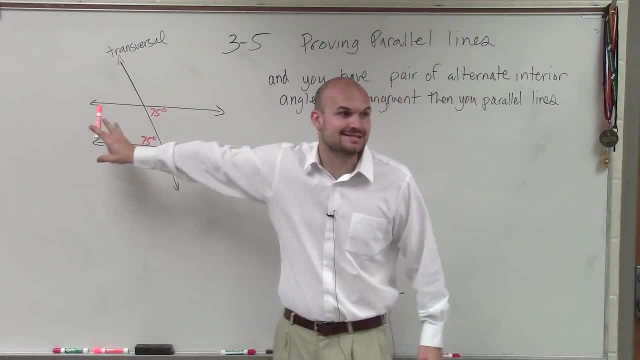 same measure. what that tells me is that I have a pair of alternate interior angles that are equal to the other two lines, Right, And what I'm trying to say by that is that the two lines are parallel. So you guys remember I told you before: don't assume angles are. 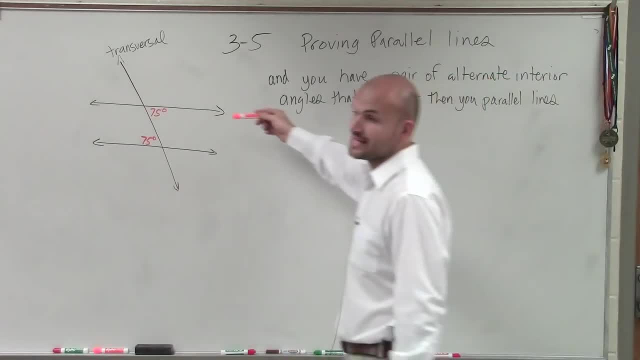 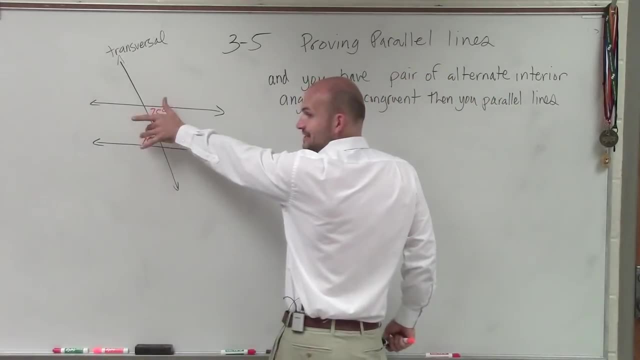 parallel, unless I tell you they're parallel or you see those nice little arrows on the lines right. Well, here's another way for you to know if you have lines that are parallel. If you see alternate interior angles that are equal, you know that your lines are parallel. 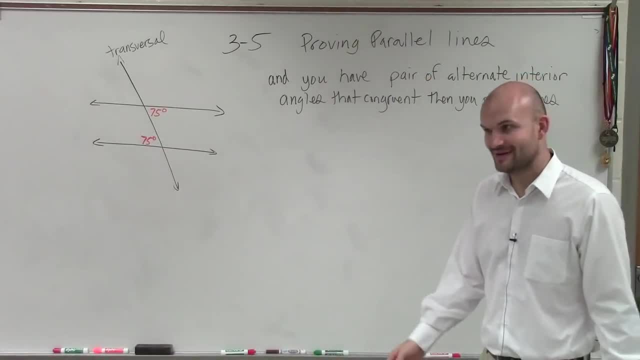 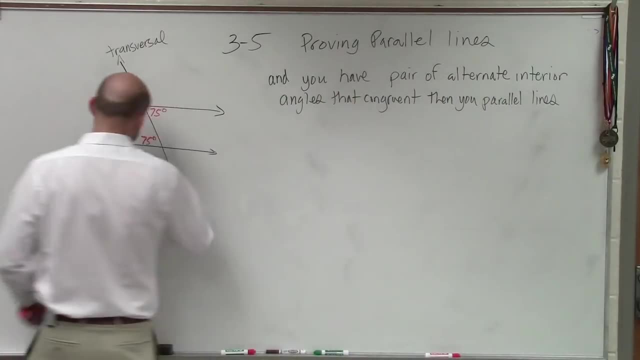 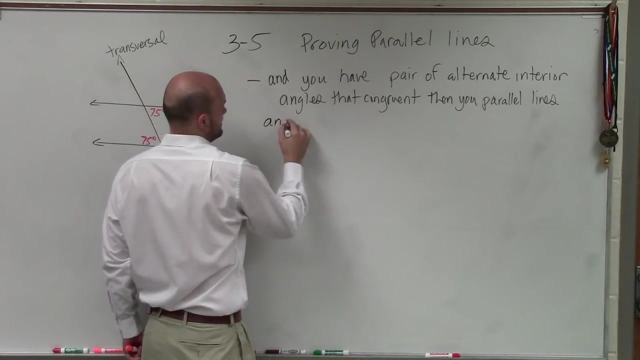 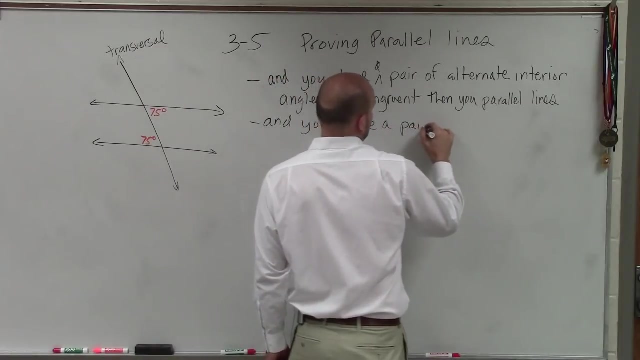 Okay, Cool, Amazing, All right. So now let's go to the next one. So let's say I have an next one. Let's say you have two lines caught by a transversal And you have a pair of consecutive. 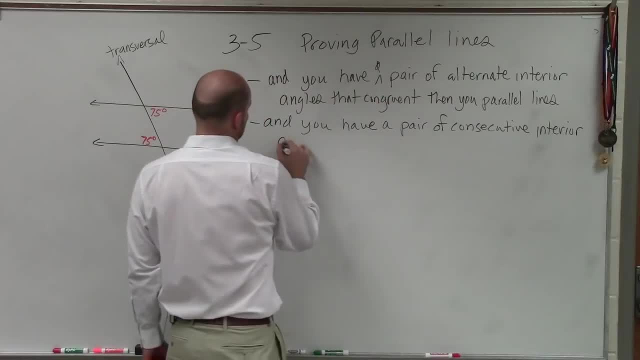 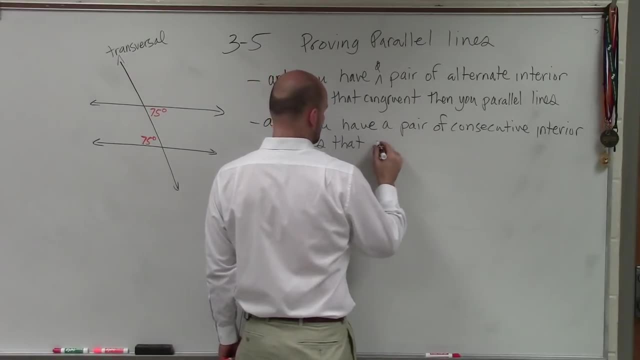 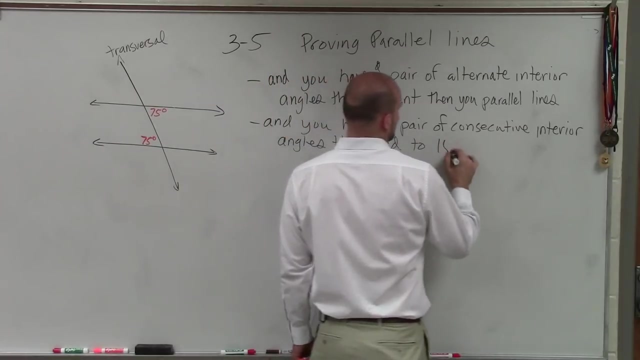 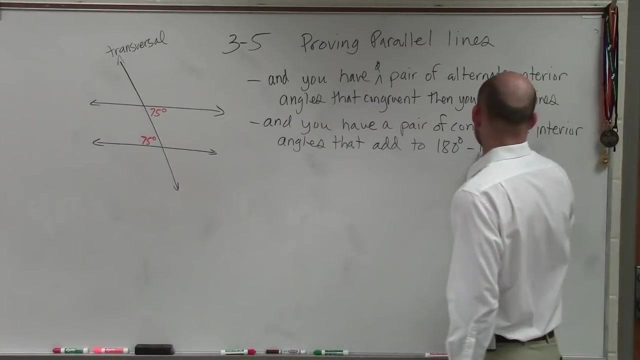 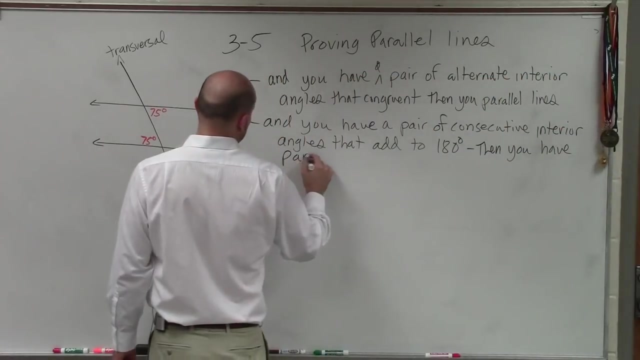 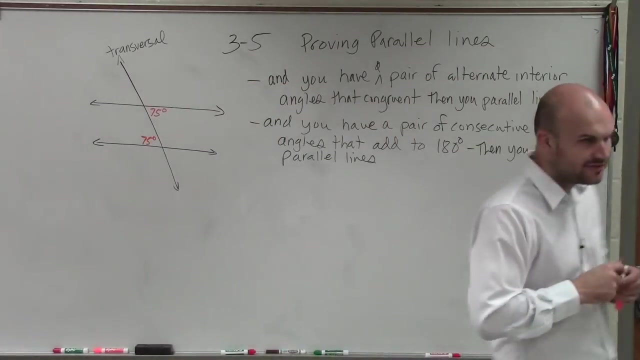 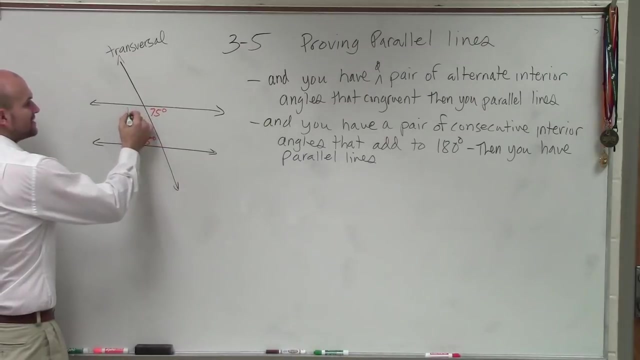 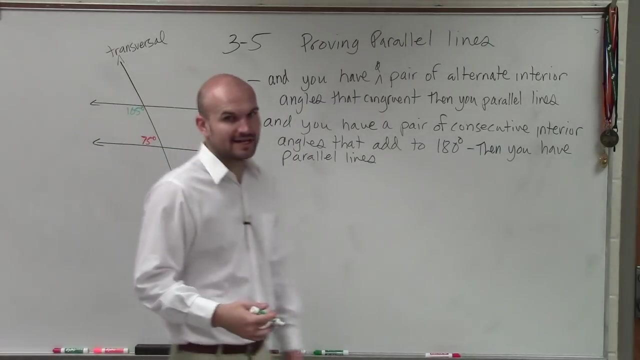 interior angles, that consecutive interior angles that add to 180 degrees, Then you have parallel lines. Okay, So consecutive interior. What exactly, again, is consecutive interior? What if I had 105 and 105 degrees? All right, Those are consecutive interior angles. So, ladies, 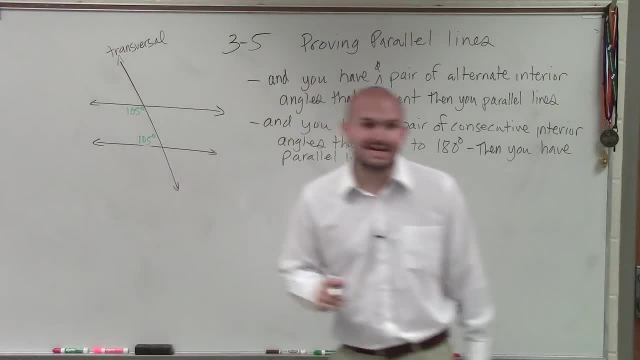 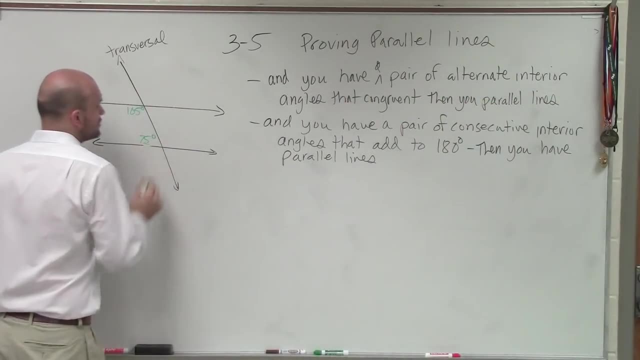 and gentlemen, if you're looking at a figure and you see consecutive interior angles, why that's not 105,, that's 75, right? If you're looking at a figure- two lines and a transversal- and you notice that you have consecutive interior angles that are supplementary, that means 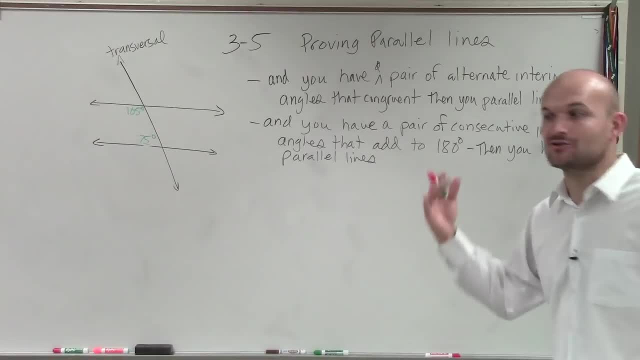 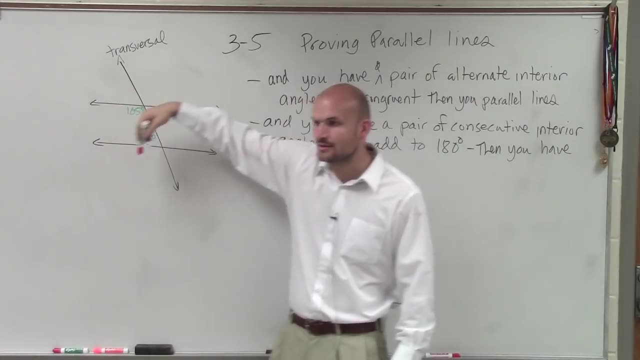 they add up to 180.. Consecutive interior angles supplementary add up to 180.. Therefore, then now, Zeth, you can say that these two lines are Zeth Wurzelman. Well, the angles are consecutive interior, and if they're consecutive interior, 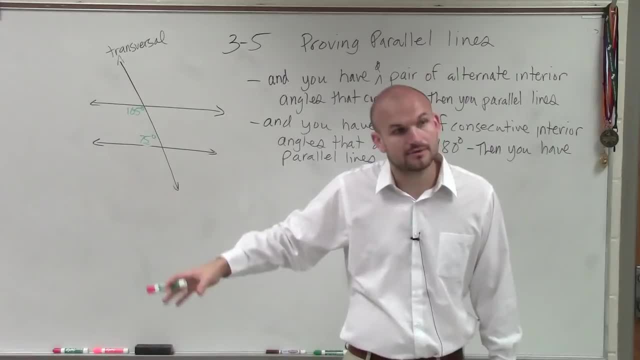 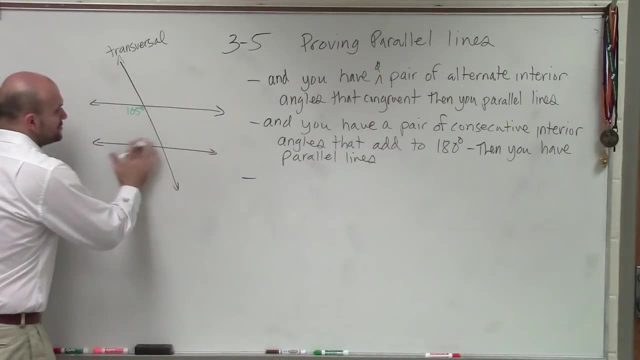 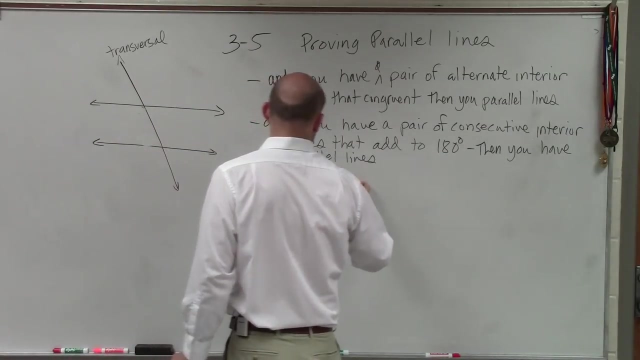 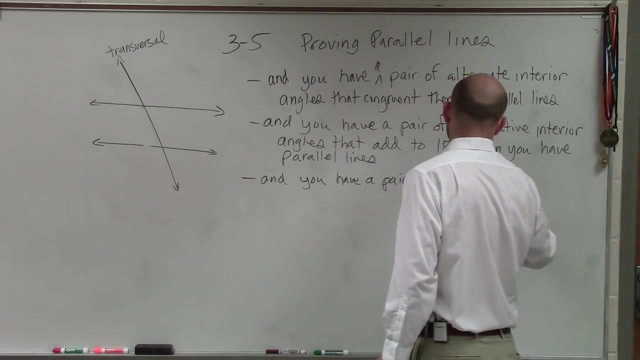 then the lines are parallel to each other. Very good, All right, Let's go. Keep on going If you have two lines caught by a transversal and you have a pair of alternate exterior angles. Speaker 1. Speaker 2.. 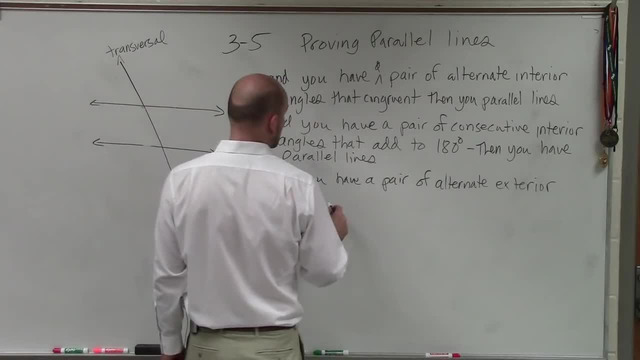 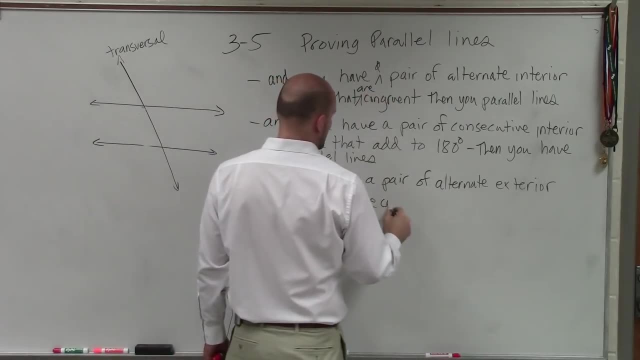 Speaker: 3. Speaker, 4. Speaker, 5. Speaker, 6. Speaker, 7. Speaker, 8. Speaker, 9. Speaker, 10. Speaker, 11. Speaker, 12. Speaker, 13. Speaker, 14. Speaker, 15.. 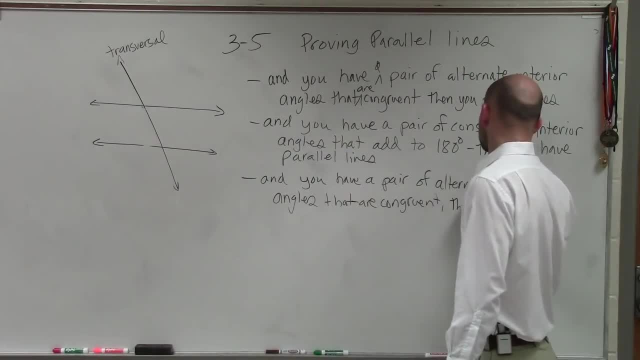 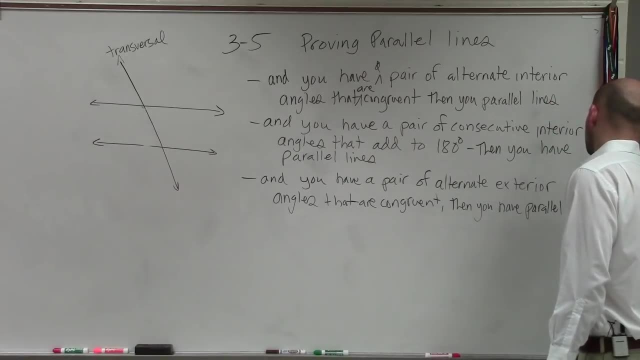 Speaker: 16. Speaker, 17. Speaker, 18. Speaker, 19. Speaker, 20. Speaker, 21. Speaker, 22. Speaker, 23. Speaker, 24. Speaker, 25. Speaker, 26. Speaker, 27. Speaker, 28.. 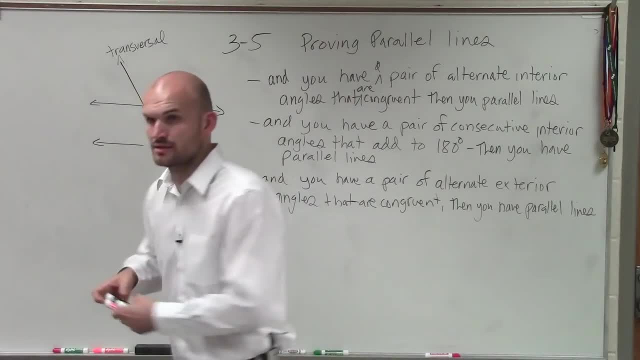 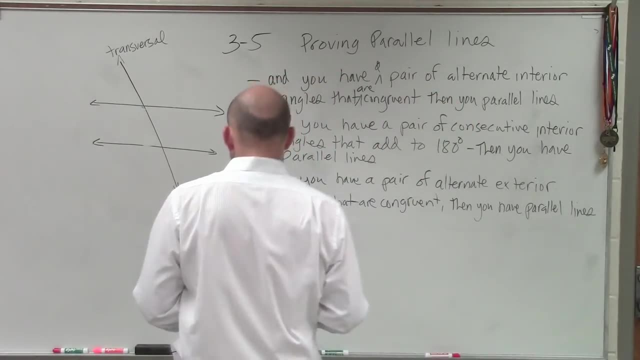 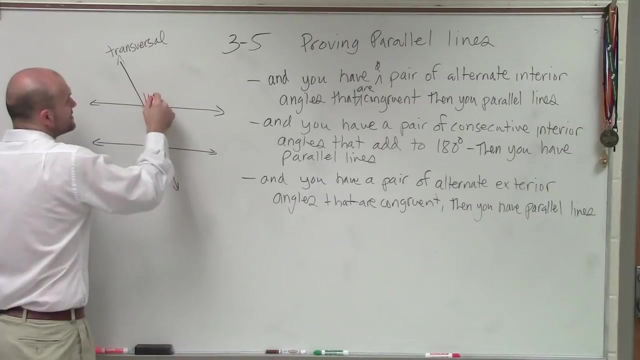 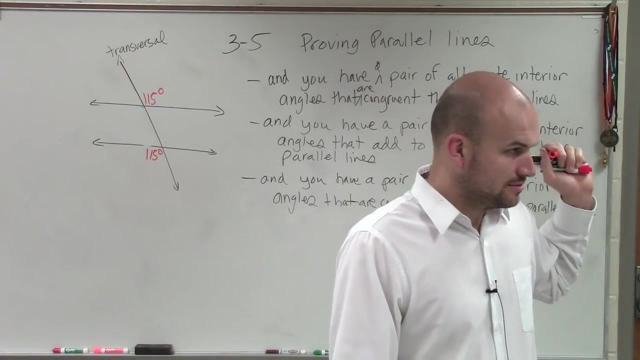 Speaker 29. Speaker 30. Speaker 31. Speaker 32. No, she's OK. Consecutive exterior angles. What about if I said this one was 115 degrees and this is 115 degrees Asia? can you confirm those are alternate exterior angles. 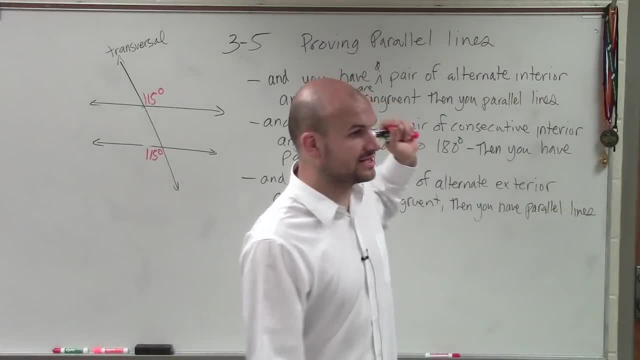 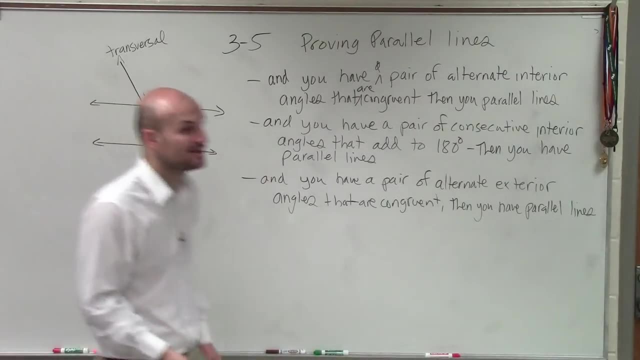 They're both exterior right And Sam, they alternate the transversal right. They're on both different sides of the transversal. So therefore you guys can confirm these are alternate exterior angles And they're equal in value right.